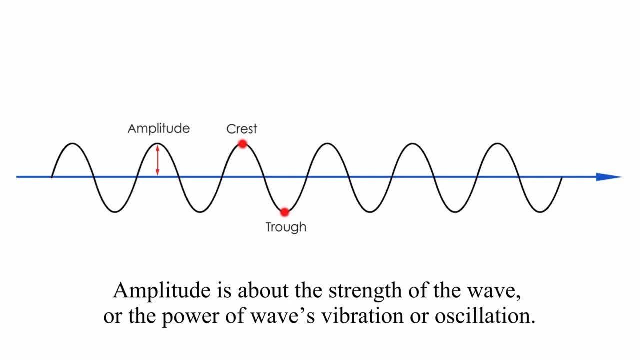 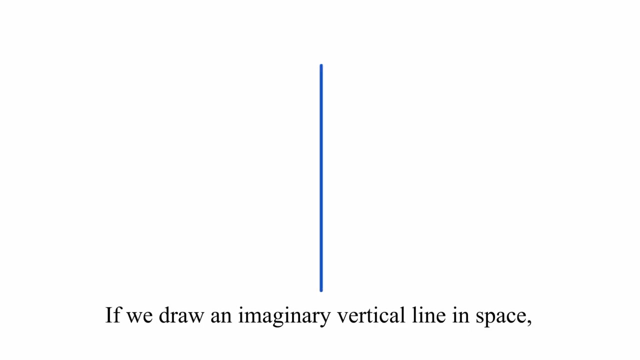 Amplitude is about the strength of a wave or the power of a wave's vibration and oscillation. In other words, the greater the amplitude of the wave, the more energy it carries. Then what's the frequency If we draw an imaginary vertical line in space? 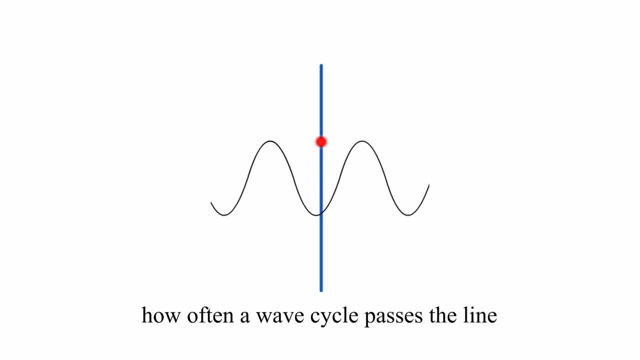 the frequency of a wave is how often a wave cycle passes the line within a certain time, for example, within one second. We can also define frequency as the number of times a wave cycle repeats within a certain time Phase specifies the location of a point within a wave cycle. 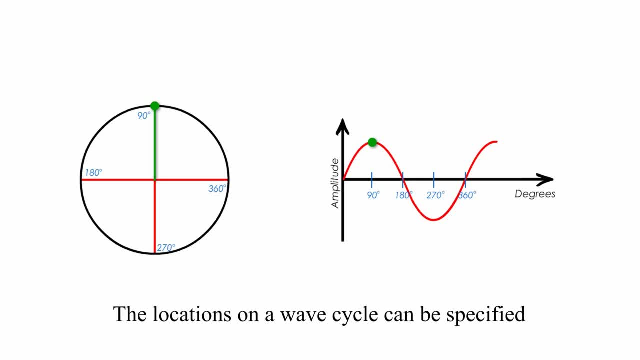 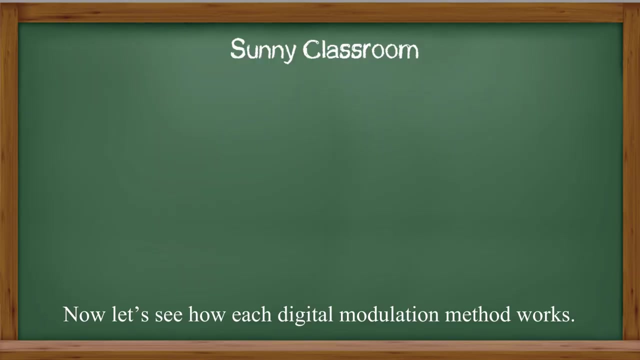 The locations on a wave cycle can be specified as an angle, in either radians or degrees, as well as in fractions of a cycle. This can be visualized with a rotating wheel and a spoke tracing the wave as time goes. Now let's see how each digital modulation method works. 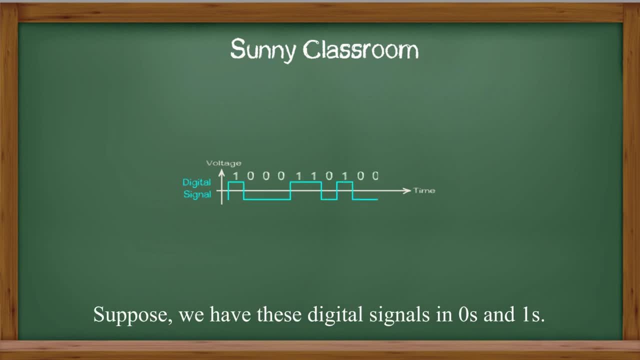 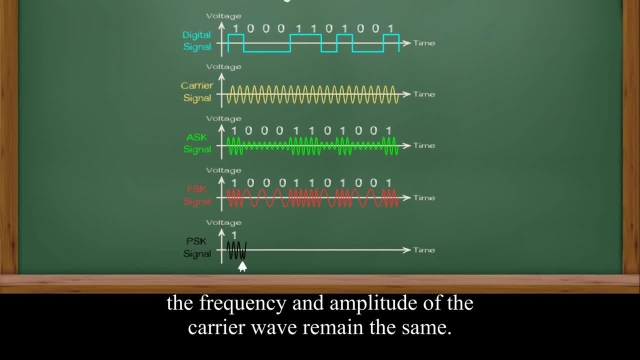 Here is the carrier wave we will use to send these digital signals. We can see from the animation: the frequency and amplitude of the carrier wave remain the same. Only change is phase, Specifically phase changes at the point where the binary value 1 changes to binary value 0,. 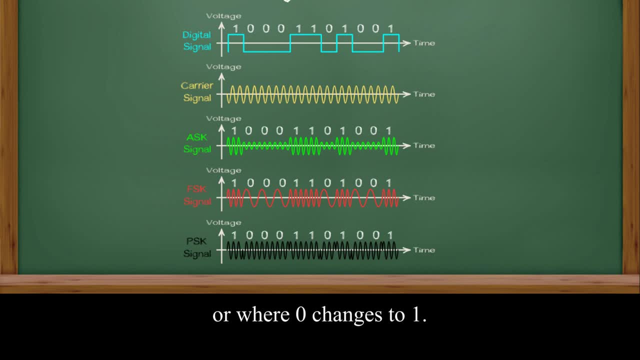 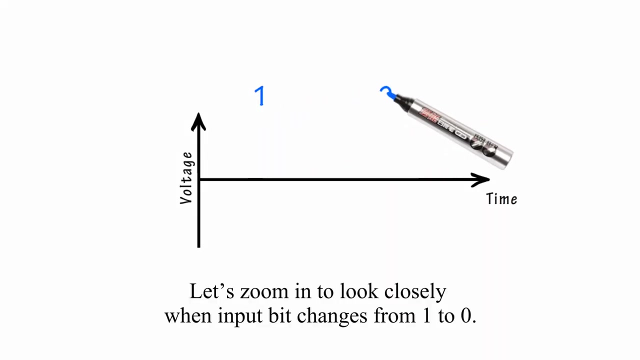 or where 0 changes to 1.. I replay this animation again. Please pay attention. Please pay attention to the turning points where the arrows flash. Let's zoom in to look closely when input bit changes from 1 to 0,, for example, 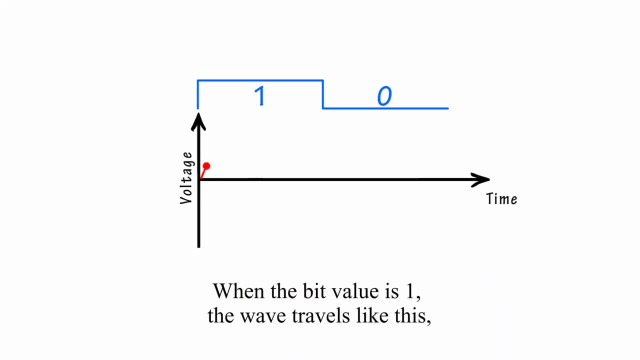 When the bit value is 1, the wave travels like this, But at the moment when the binary value changes to 0, the wave changes its direction. the wave changes its direction. It stops going up and starts going down. I hope this video is helpful. 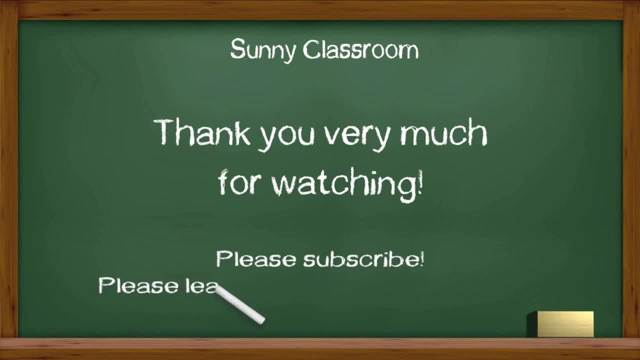 Thank you very much and see you next time. Oh, don't forget to subscribe.